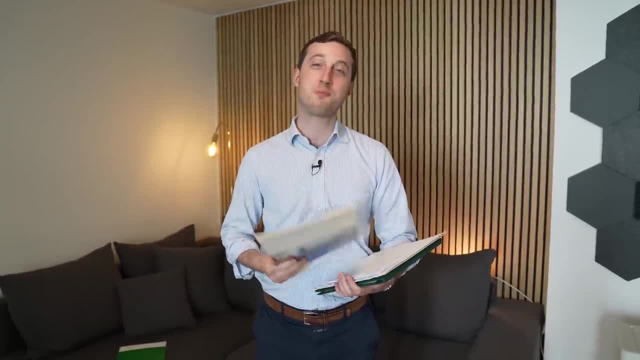 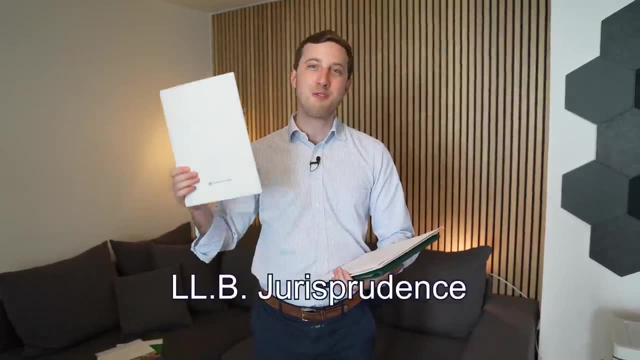 six semesters During my bachelor in business administration. I also spent a semester abroad at the university of Milan Bocconi. In the middle of my bachelor, I enrolled myself in the bachelor of law at the distance university of Hagen and later completed this as well. 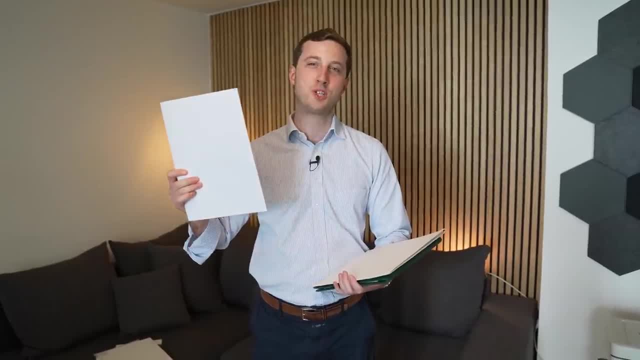 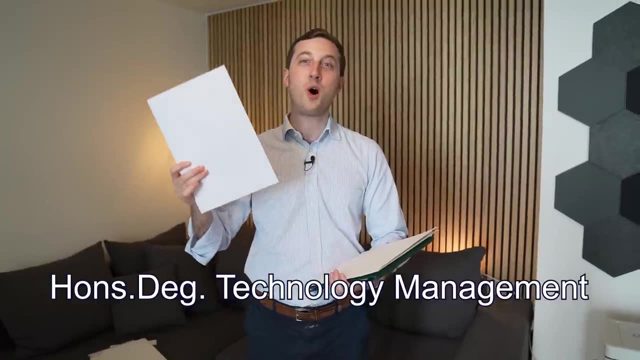 At the same time, I enrolled myself in the program of CETM, which is a joint institution of the TU Munich and LMU Munich. I graduated with the honors degree in technology management. I later enrolled for the master's degree in accounting and finance at the London School. 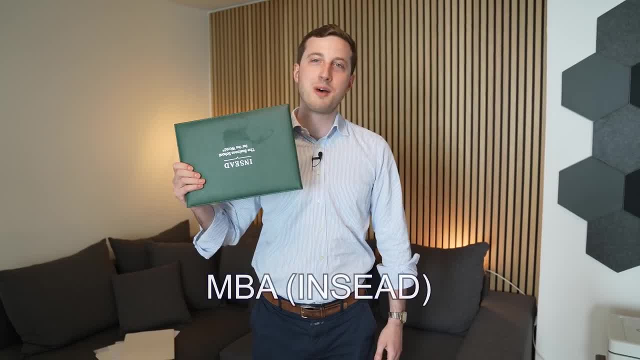 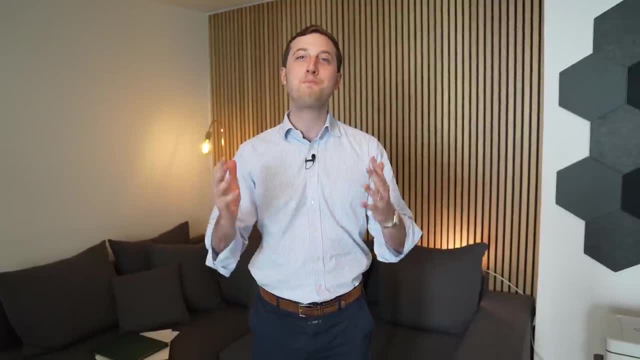 of Economics And then finally, in the end I- was¡¦d it Jump into the point- also completed my MBA at INSEAD. So in this video, I'm going to talk about exactly that. How did I do that? How did I study three bachelor degrees in parallel? And I will also share a 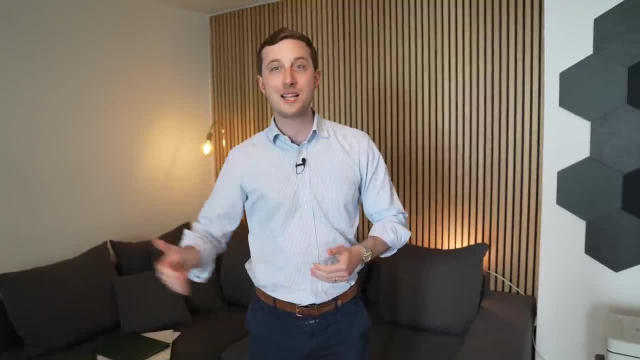 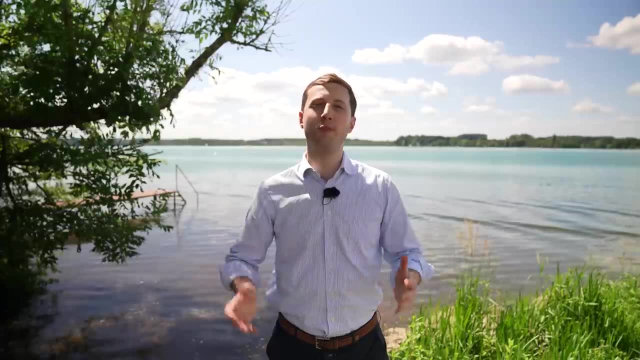 couple of tips if you intend to do something similar as well, And the last will reflect whether this actually helped myself in my career or not. So let's get out and let's get going. It's a beautiful weekend here in Munich. Today, we are visiting some of the Munich lakes. 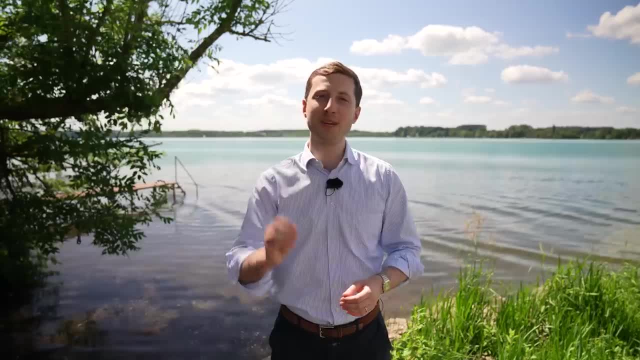 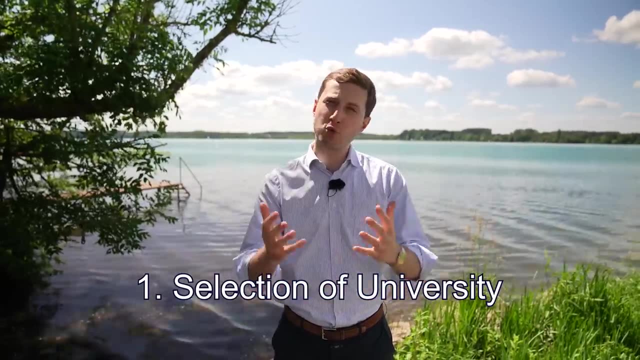 So let me share a couple of considerations that you have in your mind when thinking about starting several bachelors at the same time. The first is the selection of the university. Here, especially, some private business schools might not even offer different degree programs. In many private business schools, you can indeed only study business. 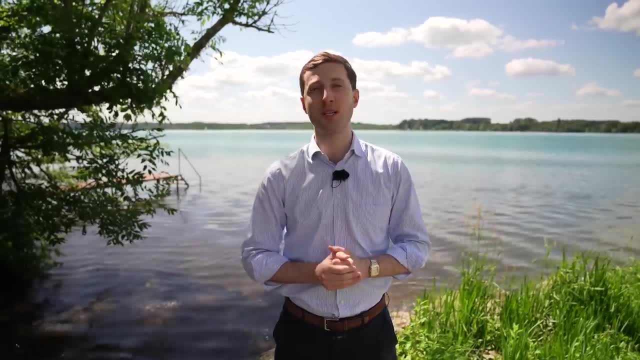 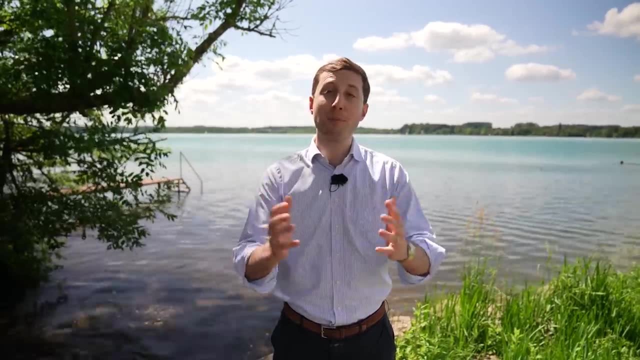 The second limitation is that often also the regulations of university sometimes do not allow you to be enrolled in several degree programs at the same time. Here in Germany it's especially the big public universities that often are a little bit more lenient. I studied at the University of Munich for my first two bachelor's. 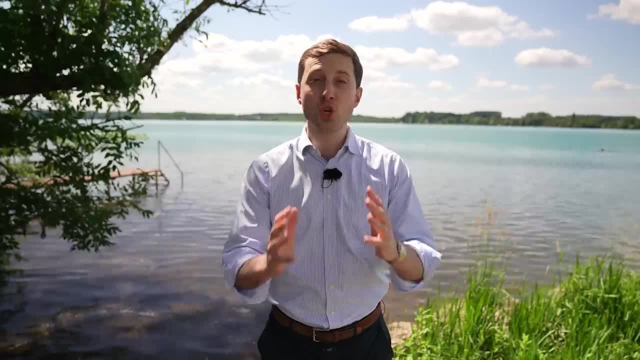 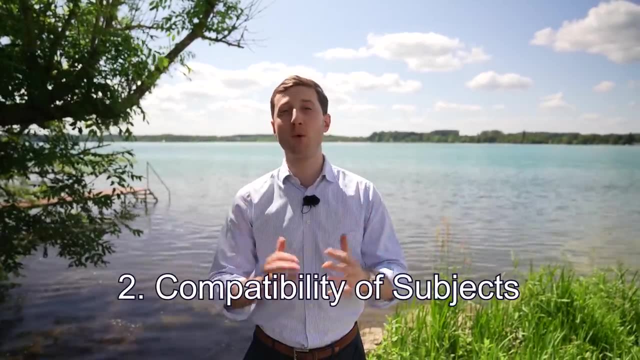 degrees and a third at a distance university. So make sure that the choice of university supports the study programs that you want to study, indeed. Second, make sure to combine subjects that are actually compatible with each other in regards to the examination structure that they have. 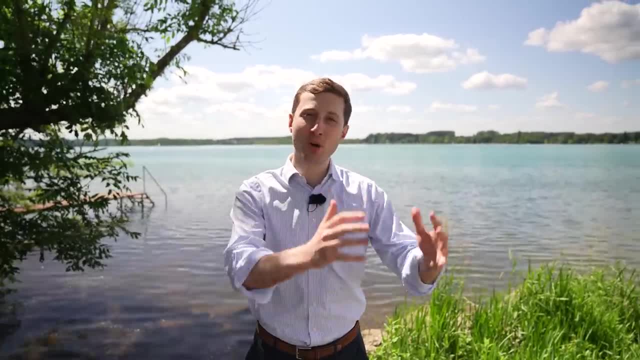 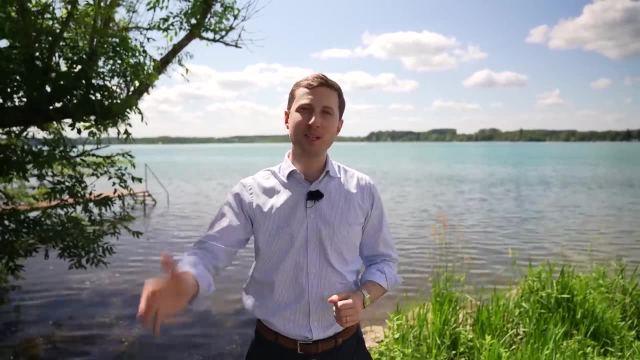 Here. one advantage of comparing, for instance, a business degree with liberal arts is that business degrees usually are very heavy on exams. So at the end of the semester you will usually have an exam period where there are lots of exams, And on the other hand, for liberal arts there are usually almost no exams at all. 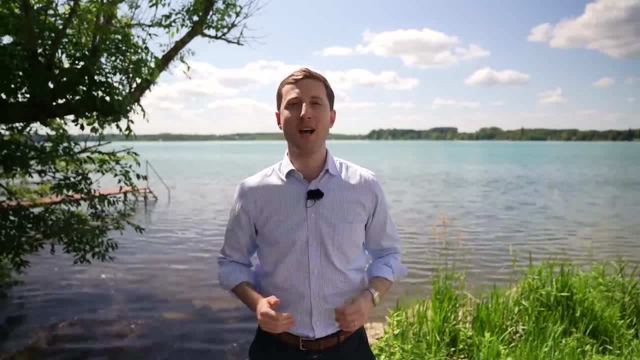 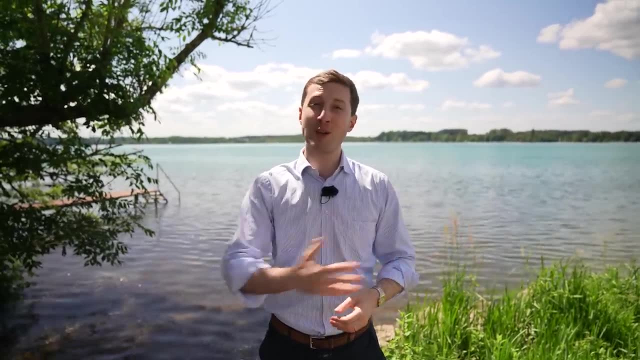 There the examination structure looks the way that you will write lots of essays, lots of written coursework that you need to prepare, and these will often need to be written during the semester. So I had the advantage that at the end of the semester I was able to just study for 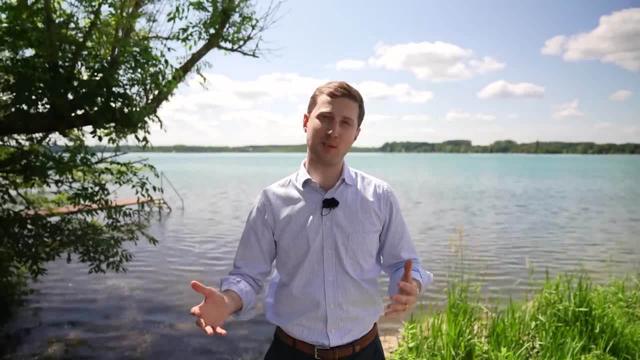 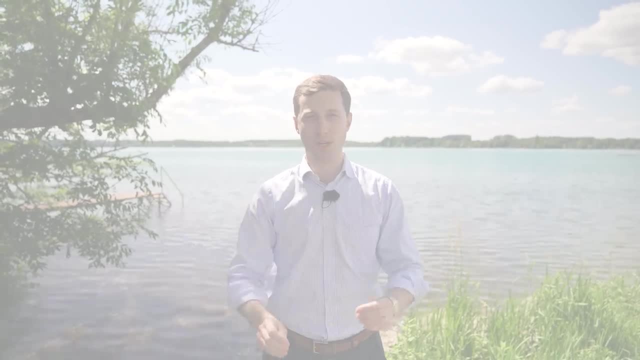 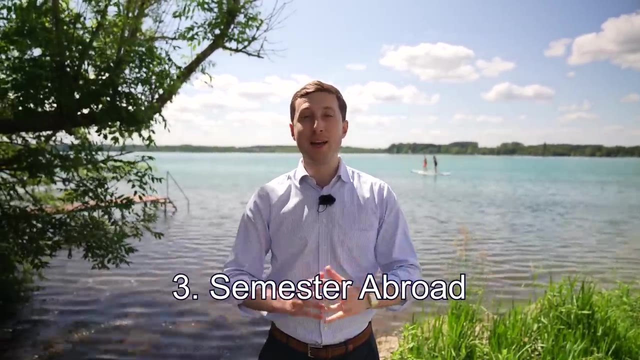 my business exams and didn't need to do that much work during the semester for this degree. And during the semester then I indeed had the time to focus for the philosophy degree and make that work. Third thing, strategically about the semester abroad. So I did a semester abroad at Bocconi University in Milan and that actually helped me to finish. my business degree earlier, because I indeed finished my bachelor in business in five semesters instead of six semesters, including the bachelor's thesis. One of the main ways how I did this is that in Milan, at Bocconi, I wrote a full exam period. 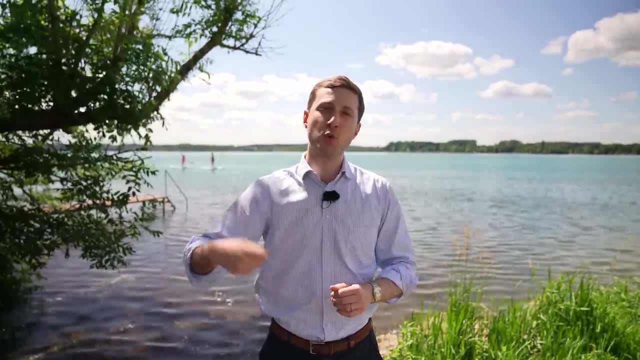 and I was able to carry over many of the exams that I wrote in Milan towards my business degree And then, once I came back from Milan, I also completed a full exam period in the second And I was able to carry over many of the exams that I wrote in Milan towards my business. 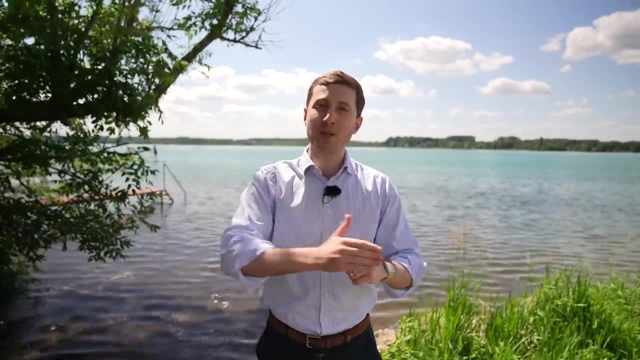 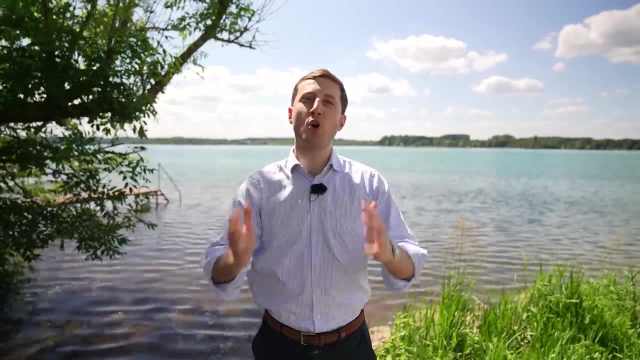 degree. I did this in the same semester in Munich as well, because there the exams happened a little bit later than the exams in Milan and still had time a couple of weeks to prepare for these exams. So I pretty much did the coursework of two semesters and only one semester. 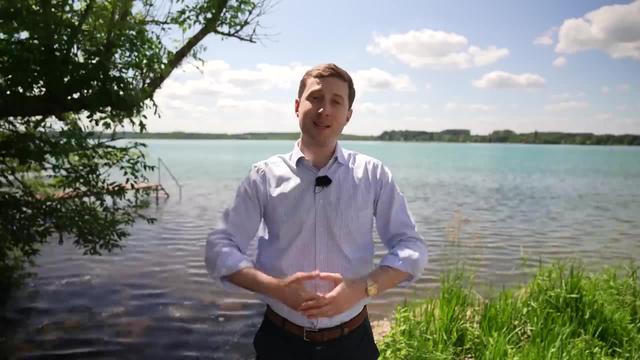 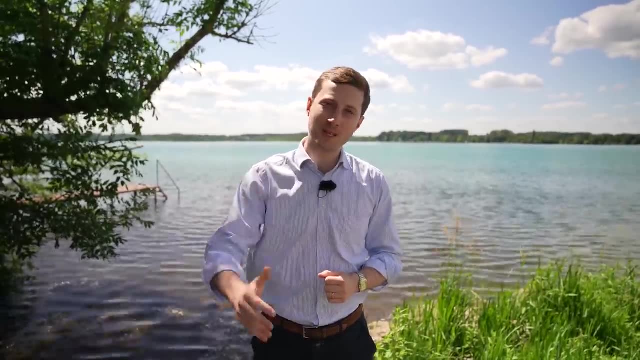 And this then enabled me to, for instance, in my last semester, complete an internship at McKinsey. This enabled me then to fully focus on my bachelor thesis in philosophy in semester number six. Many students actually extend their studies if they do a semester abroad. 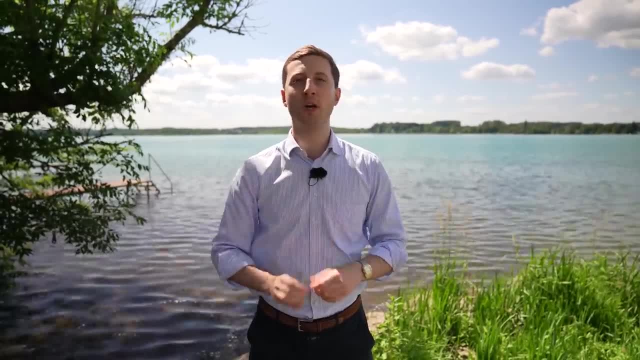 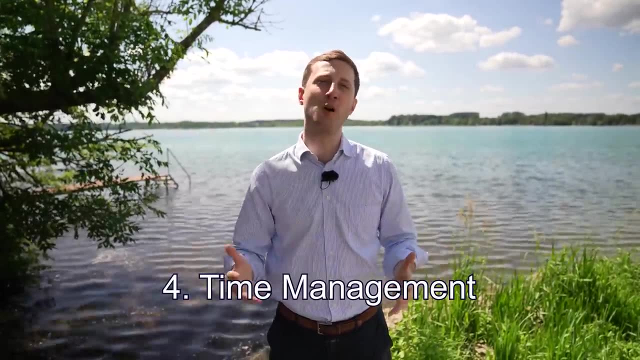 In my experience, if you set it up the right way, it can actually help you to complete your studies in a quicker way. Let's now talk about time management, because this is a topic I quite often get questions on: How did you manage to do all this? How did you manage your time? 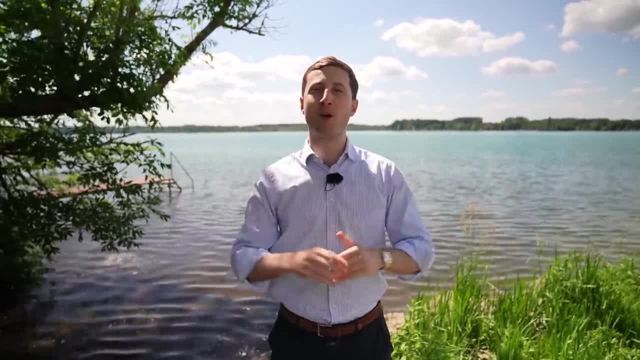 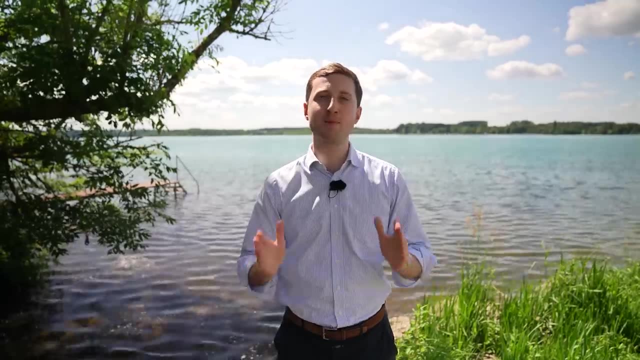 In the past I already created a video about this topic. I will link it somewhere above here. Let me also know in the comments if you would like to have more content on that. I think the basic insight is: the time management in these types of situations isn't even that challenging, If you. 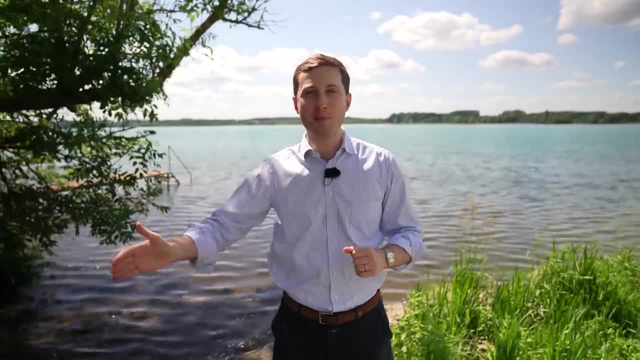 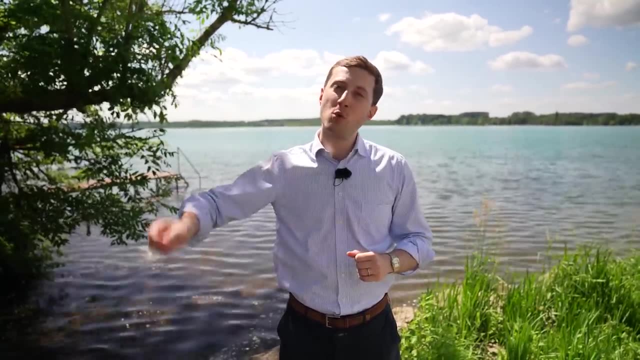 just have the pressure that on this day you will have the exam. you will make sure that the day before the exams you will do the study. If there is a coursework, an essay that you need to submit, you will make sure that in the days before you will write this essay, Because what would you? 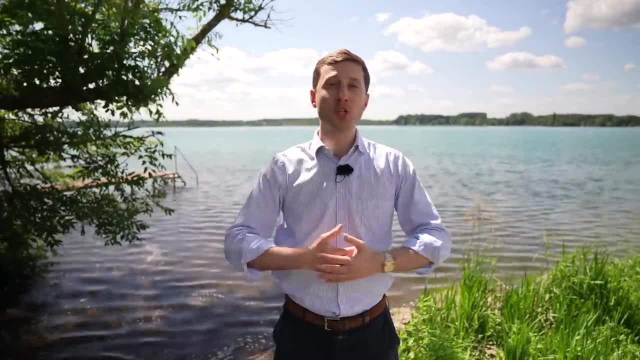 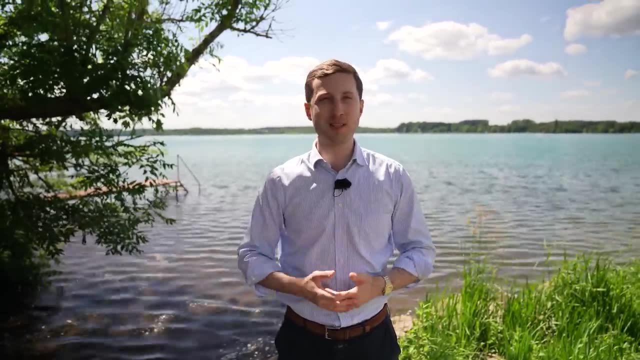 do instead, And the truth is, most people would just in the evenings, watch Netflix, hang out, maybe with some friends and so on, which, of course, can also be fun. But personally, I found that I can still do lots of these things. I still had lots of fun. 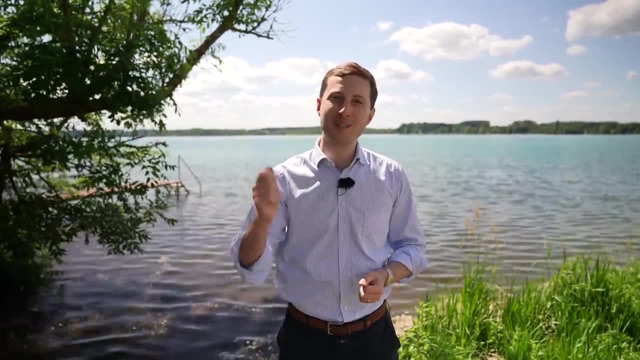 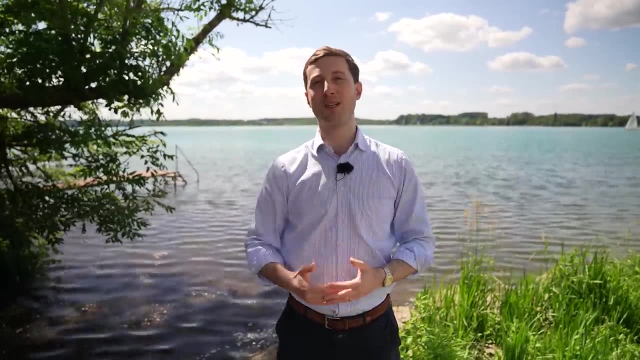 was going out with friends. But a couple of essays every semester, a couple of exams in the end of the semester. this is still very much possible if you just have the deadline, the pressure, and are just more or less focused, Forced to put in the time to not fail. So was all the effort really worth it? 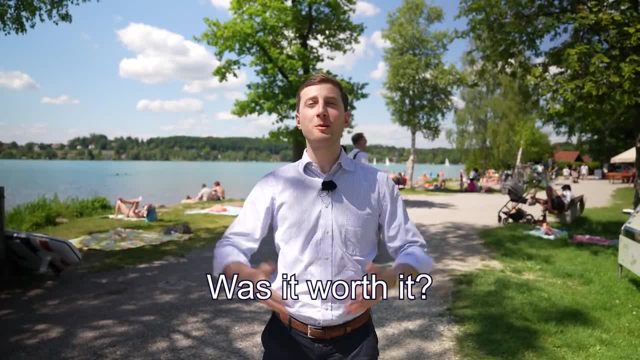 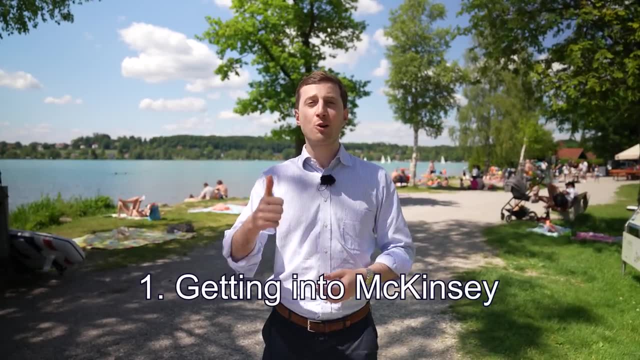 And let's look at that from three perspectives: First, to get my very first job in consulting at McKinsey. Second, for my mid to long-term career development. And third, just for my very personal life. First for McKinsey: Did this help me to get into McKinsey? And, very frankly, 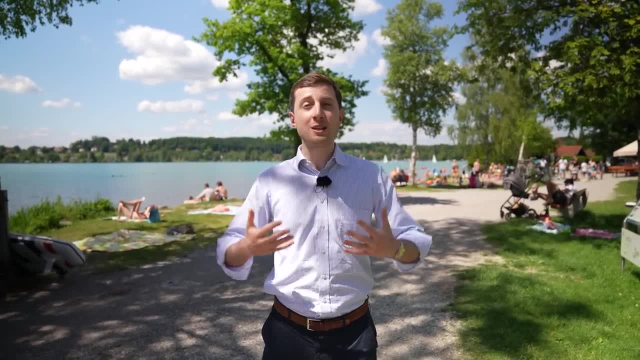 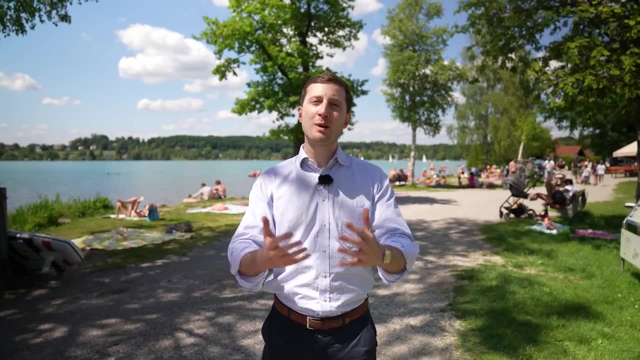 I'd say yes, it did help me. I think it was something a little bit special that I did To study both business philosophy law. Surely not all the other business candidates did that. I think, especially when you study business, it's important to have a special spike, something special that other people are. 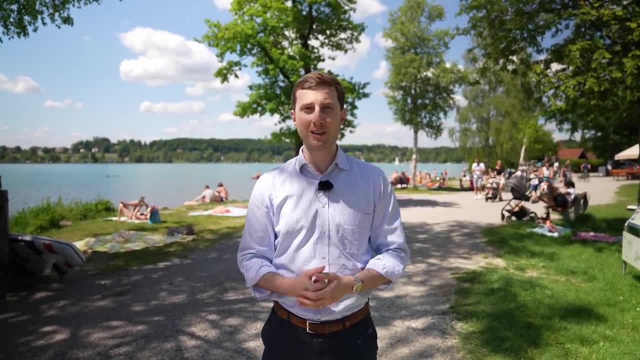 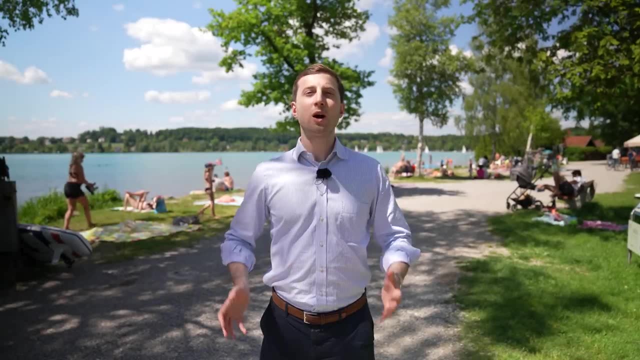 not necessarily doing, And for me I'd say that was one of the factors. Of course do not know how my profile would have been assessed if I wouldn't have done that, But for sure that did not hurt me. Second, how did this help me with my roads after McKinsey? And here, frankly, I didn't. 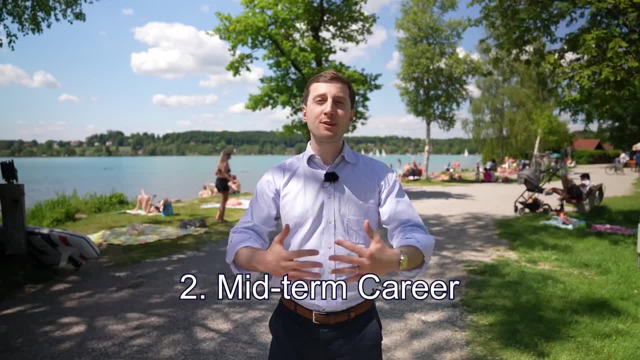 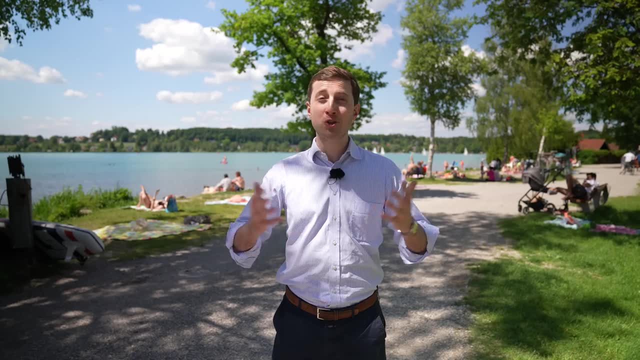 think it had that much of an effort. More or less all the things I did after McKinsey were very much based on my network personal relationships that I had up to this job. Frankly, I'm not sure if I would ever apply to any job again in the future where I would just classically with a CV in a cold. 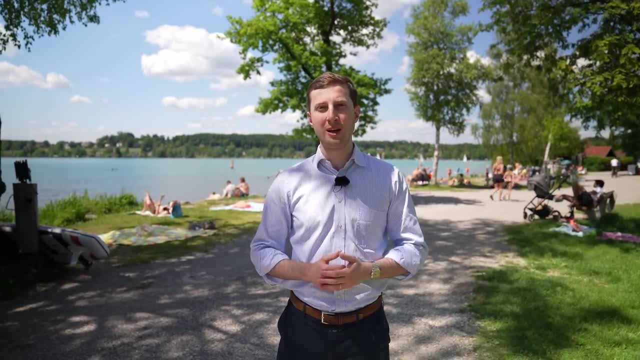 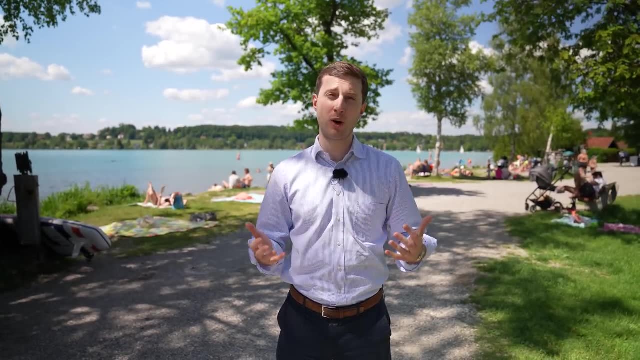 way apply somewhere. I think that's probably true as independent from your degree. I think the further you advance in your career, the less important your actual degrees will be, that you may be accomplished, attained somewhere in the past, I think at some point. it's just not that. 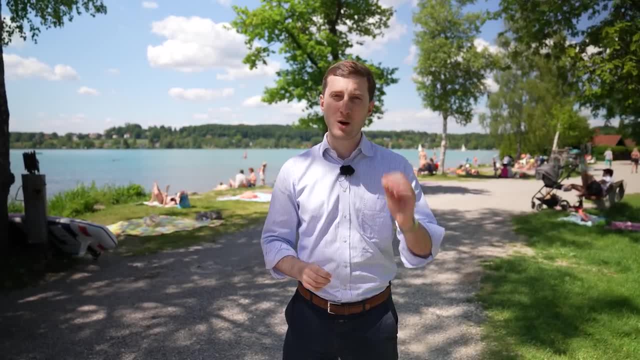 important anymore. I think it especially helps you to get in, to get that very first job. And third, how do I assess this for myself, for my personal development, for the knowledge that I built? And here, frankly, starting with the business philosophy: law, law, law, law, law law. 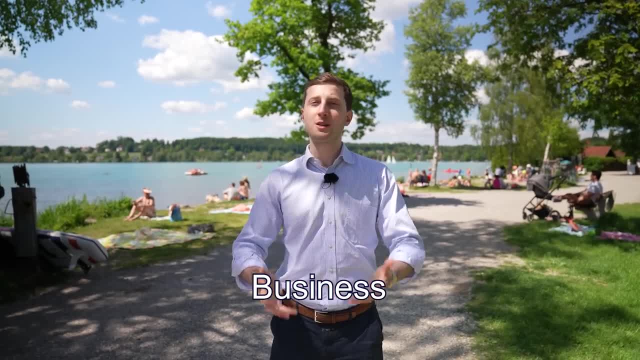 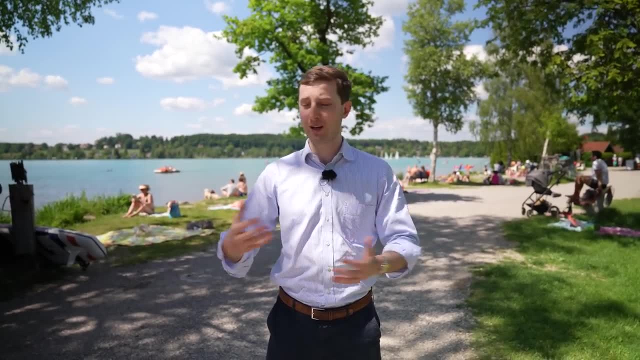 and here, frankly, starting with the business degree, spending a couple of years in management consulting will be at least as effective at starting and completing a bachelor in business. So, yes, while it helped me, of course, to get the context, understand, a couple of things, a 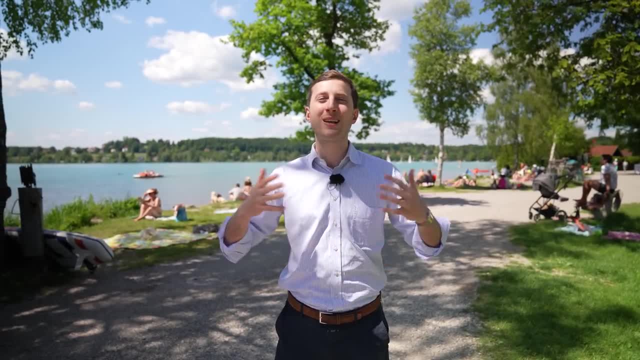 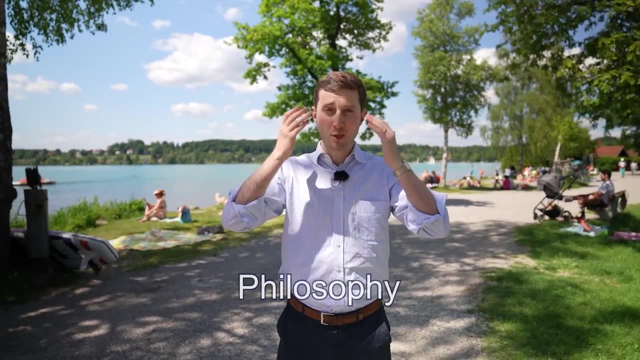 bit better just for that. probably the time in consulting alone would have done at least that much for me myself. Second, the philosophy degree. I think this very much shaped just how I approach problems, how I think about problems. I think it's just very difficult, also for myself.